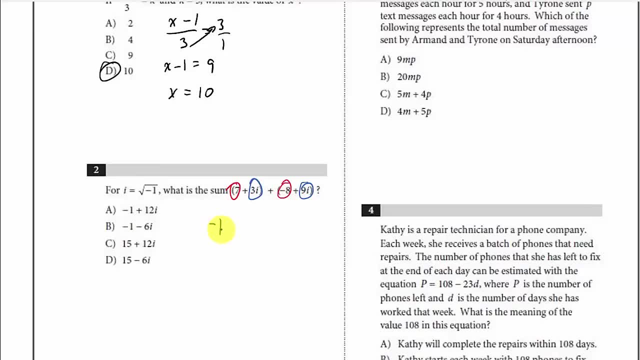 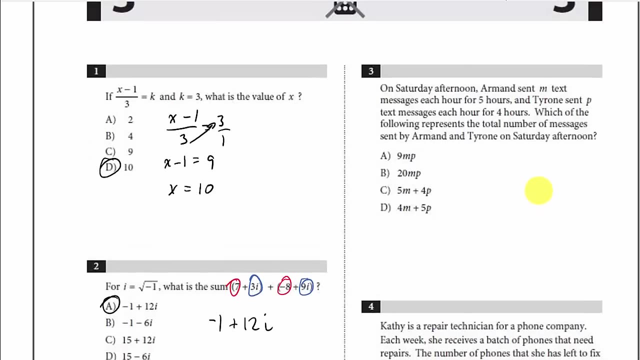 together, and so 7 plus negative 8 is negative 1, and then 3i plus 9i is 12i, and so that would give us a all right number three. on saturday afternoon armand sent m text messages each hour for five. 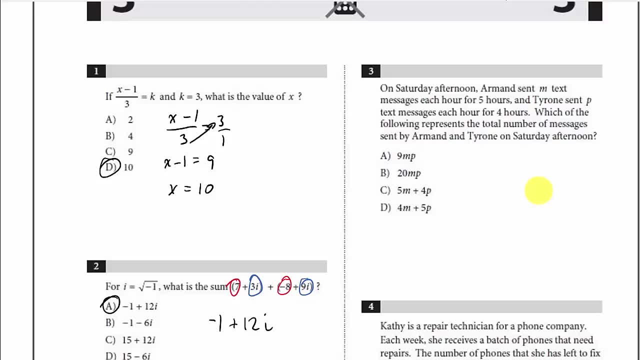 hours and tyrone sent p text messages each hour for four hours. which of the following represents the total number of messages sent by armand and tyrone on saturday afternoon. all right, so well. this one. it says: armand, you sent m text messages each hour for five hours, so m is the number of messages he sent each hour. 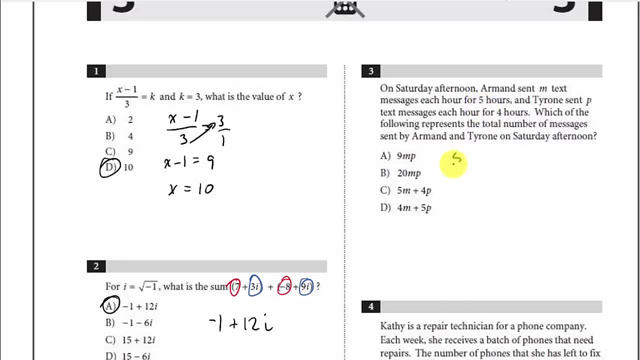 and he did that for five hours, so that would be five times m. and then tyrone sent p text messages each hour for four hours, so that would be, uh, four p. all right, four times p. and they want to know the total that they sent together, so we would add them, so that's five m plus four p. 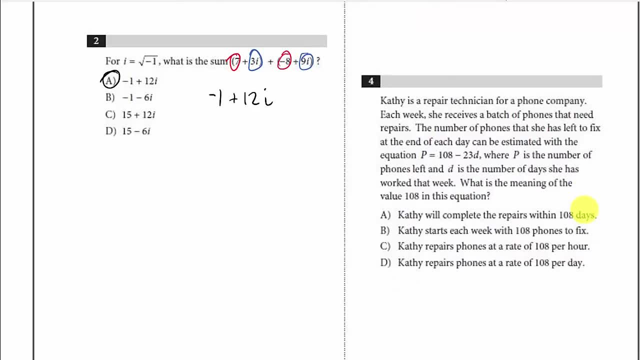 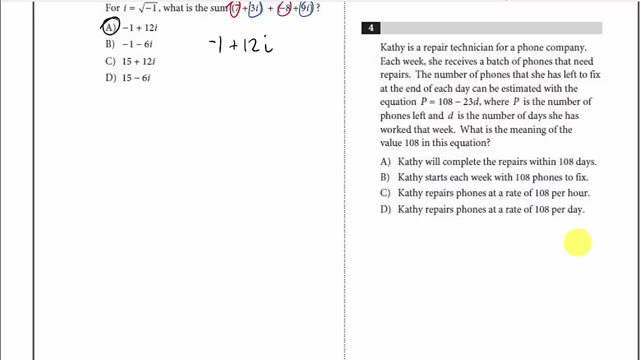 that would be c. kathy is a repair technician for a phone company. each week she receives a batch of phones that need repairs. the number of phones that she has left to fix at the end of each day can be determined with. with the equation, let's write this: p equals 108 minus 23 d, where p is the number of phones left. 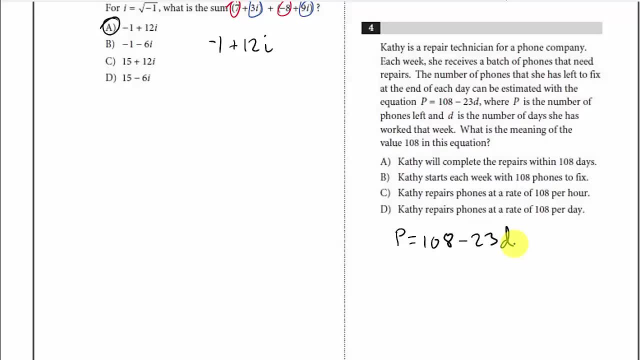 and d is the number of days she has worked that week. what is the meaning of the value of 108 in this equation? well, let's see we're doing 108 and let's see the what is d? all right, where p is the number of phones left and d is the number of days she has worked that week. 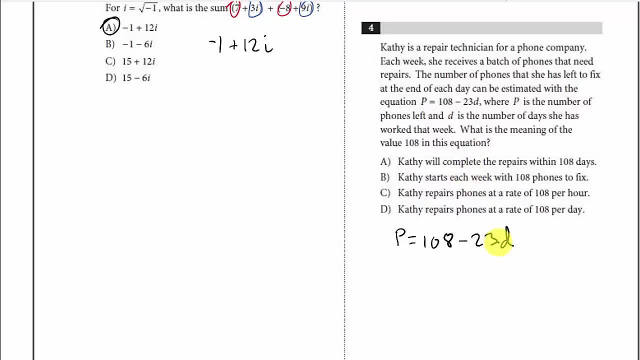 all right, so we do the 23 times d. well, that would that would be b. kathy starts each week with 108 phones to fix. okay, so, because p represents how many she has left. so if we take the number she started with minus how many she fixed, then that would be. that would leave us with how many. 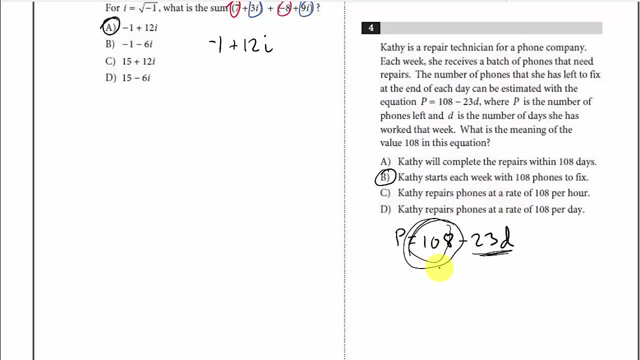 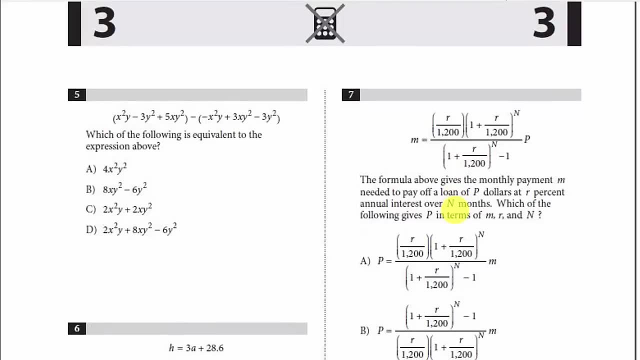 she has left, so this has to be how many. she started with all right, all right. which of the following is equivalent to to the expression above all right? so all this is is just combining like terms. now, let me say this a lot of times: it's harder to subtract than it is to 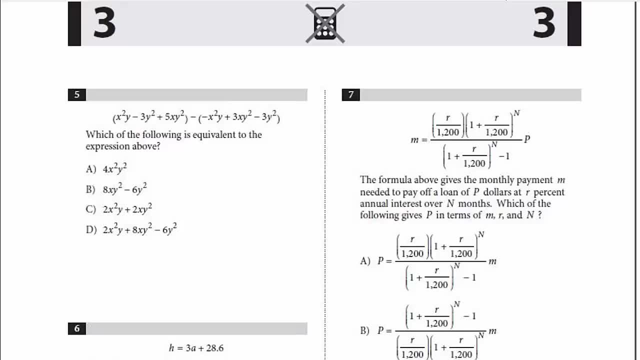 add, and it may take, you know, one extra step, but you're less likely to make us make a mistake. what i would do here is: uh, rewrite this and change this to a plus, and then remember: if you change this up to a plus, then you have to. 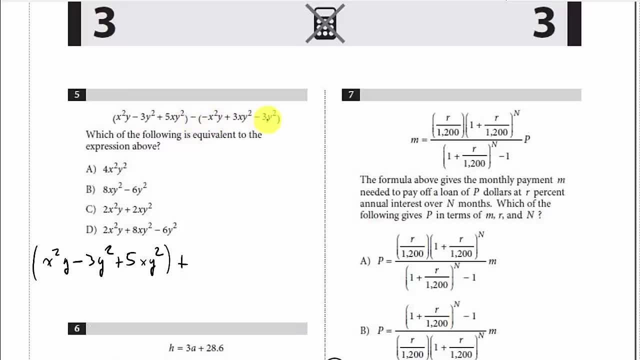 change the sign of each term inside the parentheses, so that would be x squared. y plus 3xy squared, i'm sorry, minus 3xy squared plus 3y squared. and then you just combine like terms so that would be: and then you just combine like terms, so that would be this one and this one, that's 2x- y squared. 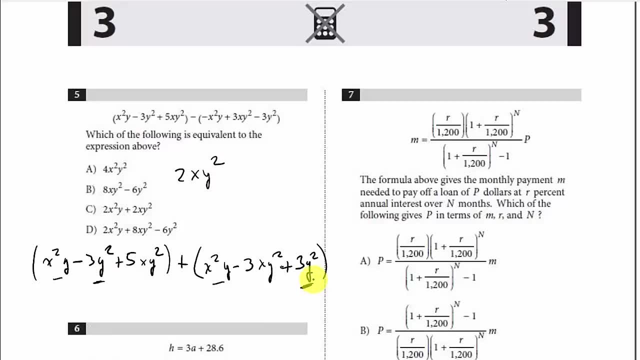 and then we've got a y squared here and a y squared here. well, that just goes to zero, the negative 3y squared plus 3y squared, and actually we could stop there. we would know it's this one, because we're only going to have two terms. but let's look at this. so we got 5xy squared. 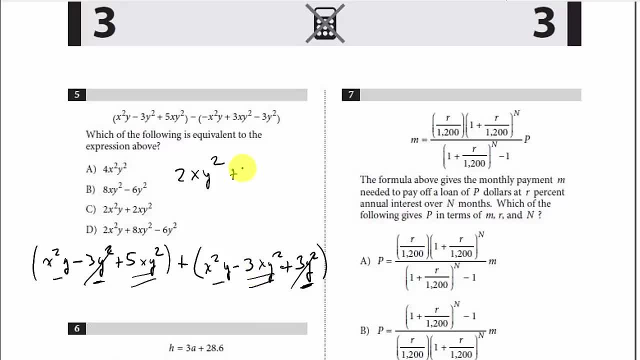 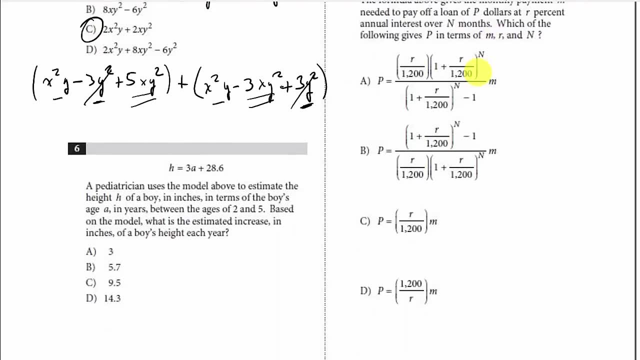 3xy squared, 5 minus 3 is 2, so that's 2 x y squared, and so that would give us c a pediatrician. a pediatrician uses the model above to estimate the height h of a boy in inches, in terms of the boy's age a in years between the ages of two and five. 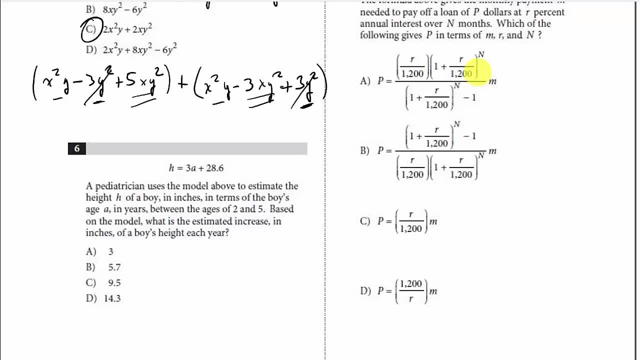 based on the model, what is the estimated increase in inches of a boy's height each year? now, don't let the two and the five throw you off, okay, you don't need that. we want to know what's the, what's the increase in height? okay? well, if you look at this, the slope of the line, your slope. 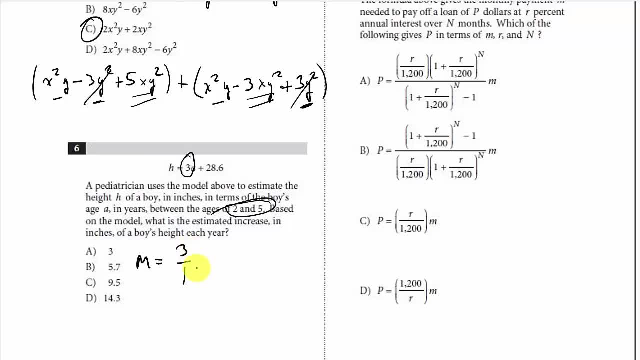 is three over one. so remember, this is rise over run, so the run that's. see, if you plot this, this is a and this is H. okay, so that's the age. so if we go over one year, well, we're going up three inches and so that would be three. all right, so, hopefully, hopefully. 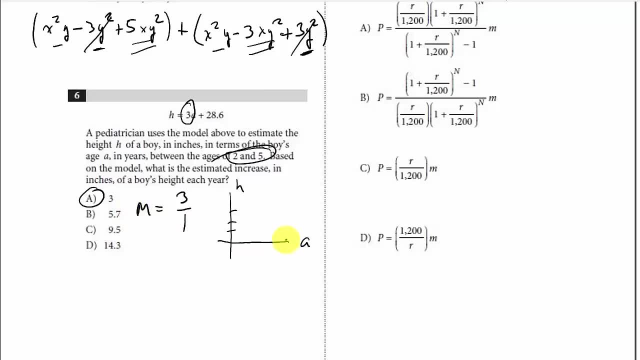 that one made sense, okay, because one tells us how we move left and right and we're just using, we're just moving one year, and for every one year we move to the right, we're moving up three, and so the change in the years is, I mean the- 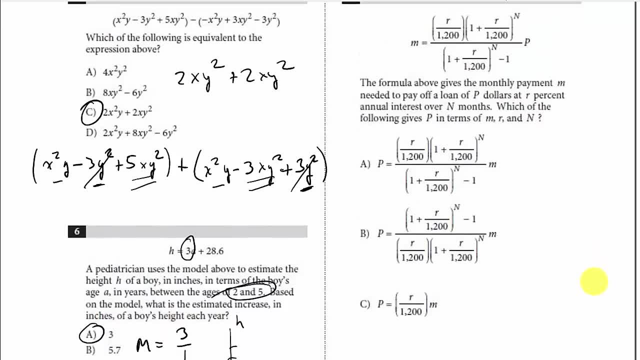 change in the height is three. all right, so let's look at this. when the formula above gives the monthly payment M needed to pay off a loan of P dollars at our percent annual interest over in months, which are the following: gives P in terms of M are in in. well, this one's easy, we're. all we're doing is solving for P. 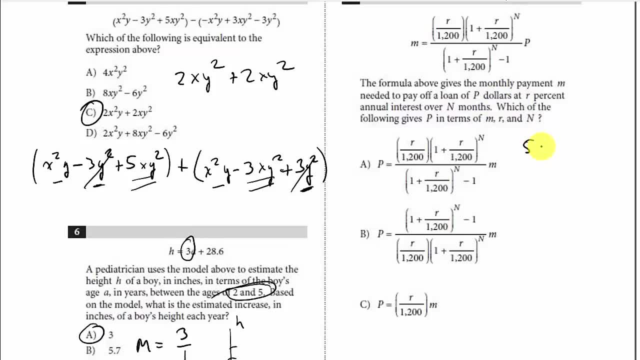 and that's kind of like. if you had something like this: five equals E, three-halves X. see, we're just solving for P, just like here we would be solving for X. what do you do? you multiply by the reciprocal. so this would be just be. 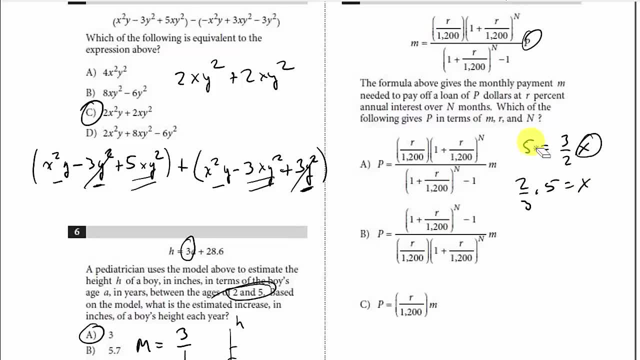 two-thirds times five equals X. so that's the same thing that we're doing here. we're just doing the reciprocal of this and multiplying it over here, and so you don't even need to write it down. what is this when you flip it? well, this goes. 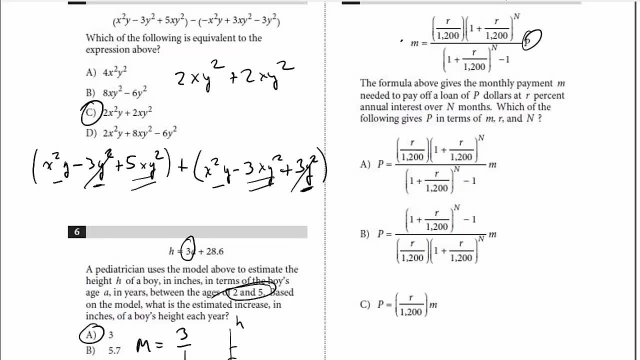 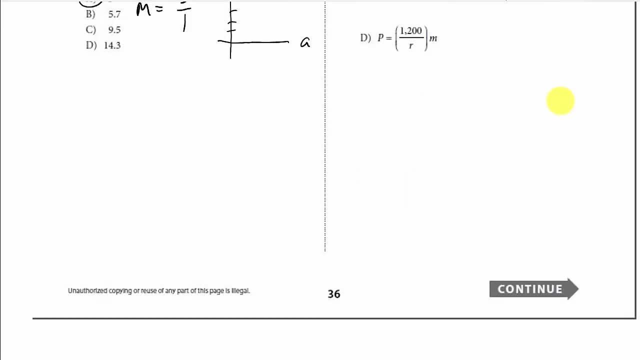 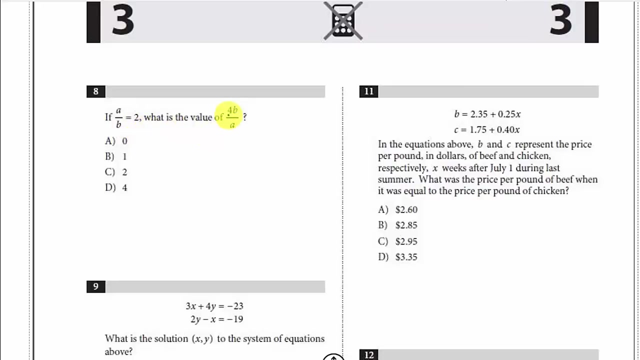 into the numerator. let's see which one have. that one has that in the numerator. well, let's see this one doesn't. uh, let's see this one. that one does. and then there's the numerator and the denominator here. so it would be alright. so how about this one we got? A over B is equal to two. what is the value? 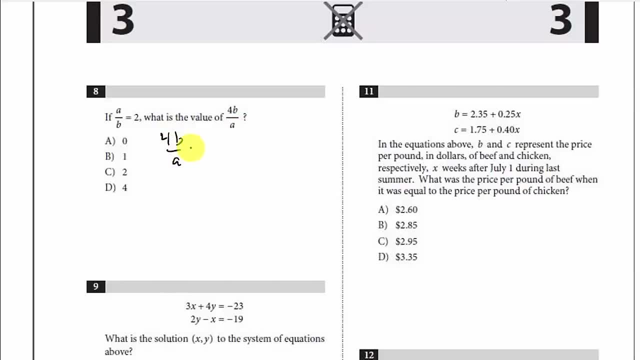 of four B over A. well, the first thing I noticed here: four B over A, that can be four times B over A. We can split them up like that. Well, over here we've got AB. Well, these are just reciprocals. So if AB is equal to two, then B over A is equal to the reciprocal of this. 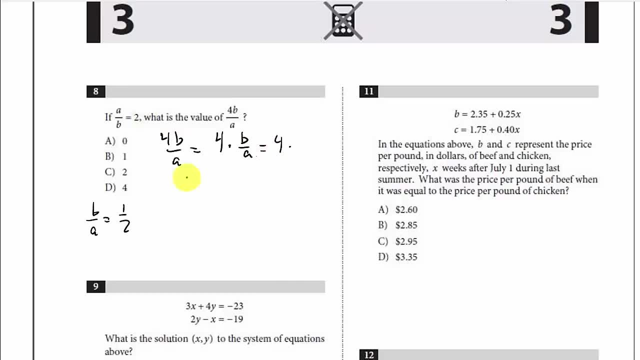 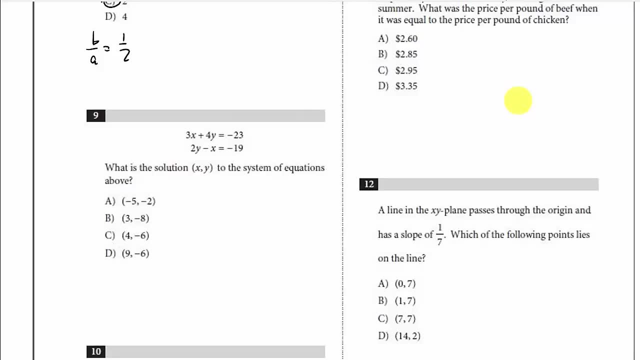 which is one half, and so this is four times. and B over A is one half, and that would give us two, which is C. What is the solution XY to the system of equations? All right, so one thing you could do is you could just start plugging in and, you know, see where you see which ones work. but I think 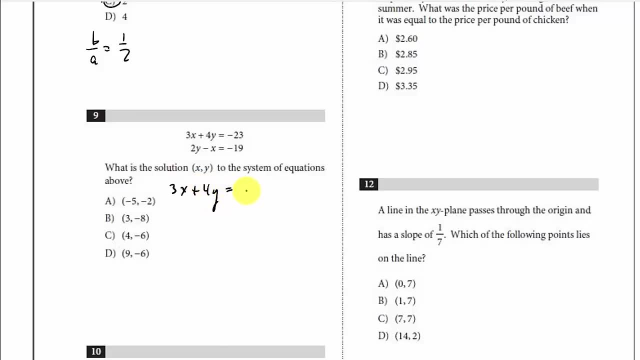 it'd be quicker to do the 3X plus 4Y equals negative 23, and then write this with the X and Y swapped, So that's negative. X plus 2Y equals negative 19. And then you can solve this using addition method. So we would multiply by negative 2.. 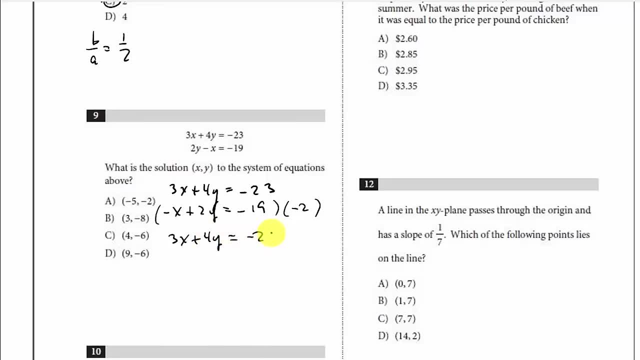 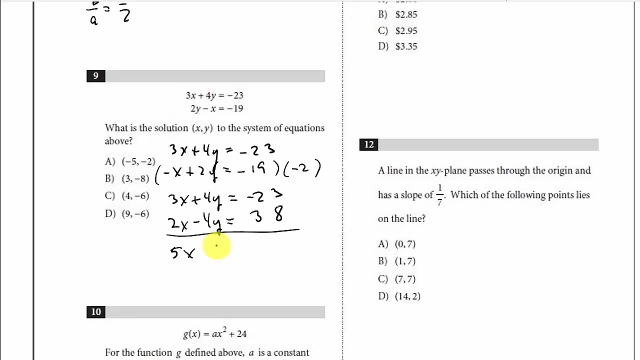 So that's 3X plus 4Y equals negative 23. And then that would give us 2X minus 4Y equals 38. Okay, and then if we add these, we get 5X is equal to 15.. X equal 3. And they want us to. 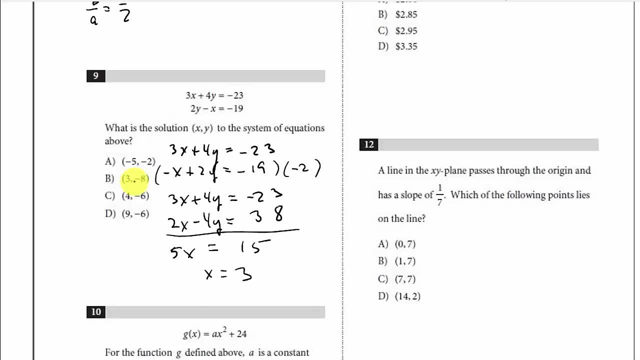 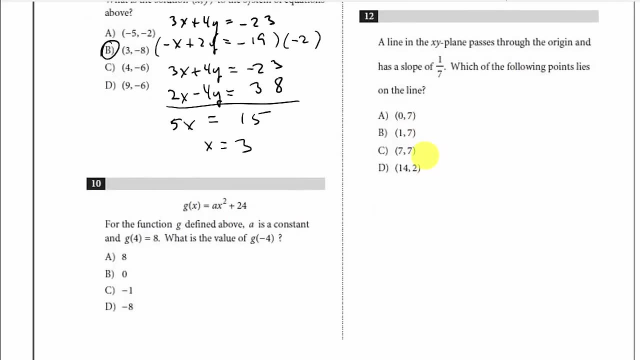 find the solution. but look, we've got x equal 3.. This is the only one where x is equal to 3, so we can stop there. That's b For the function g defined above. a is a constant and g of 4 is. 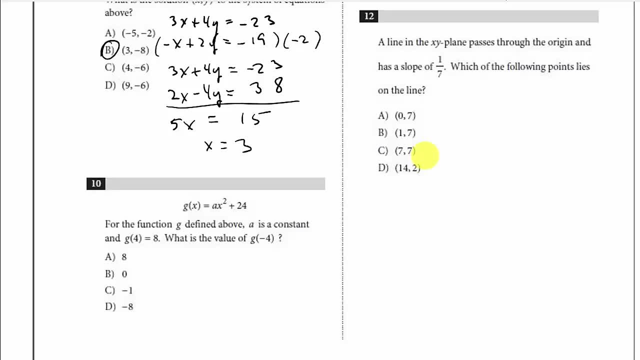 equal to 8.. What is the value of g of negative 4?? So what we need to do first is figure out what a is. So we know that g of 4 is equal to a times 4 squared plus 24, and that equals 8.. See, I've just. 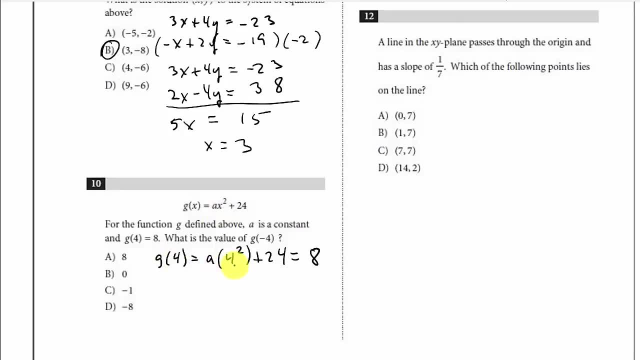 plugged the 4 in for x, And so this gives me 4 squared is 16, so 16a plus 24 equals 8.. And then all I need to do is solve for a. So I get: 16a is equal to negative 16.. a is equal to negative 16.. 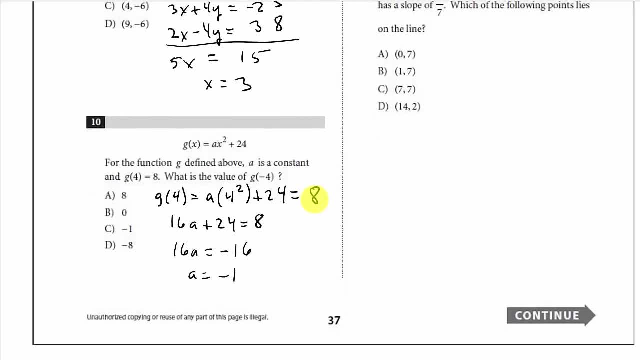 a is equal to negative 1.. And so now that's going to give me: g of x is equal to negative x squared plus 24.. And then I'm going to plug the negative 4 in, So g of negative 4 is equal to negative. 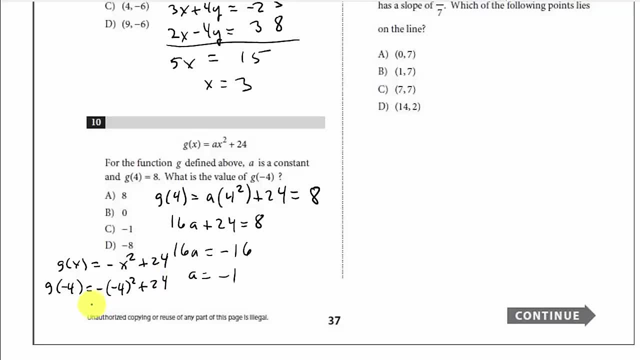 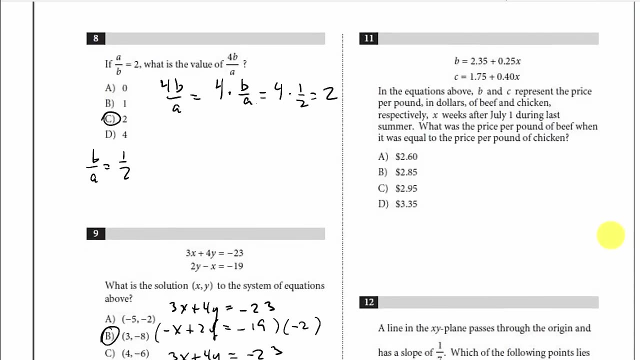 negative 4 squared plus 24.. And so that's going to be. that's the negative. Negative 4 squared is 16 plus 24.. And that is going to give us 8.. So our answer is a, All right. in the equations above, b and c represent the price per pound and dollars of 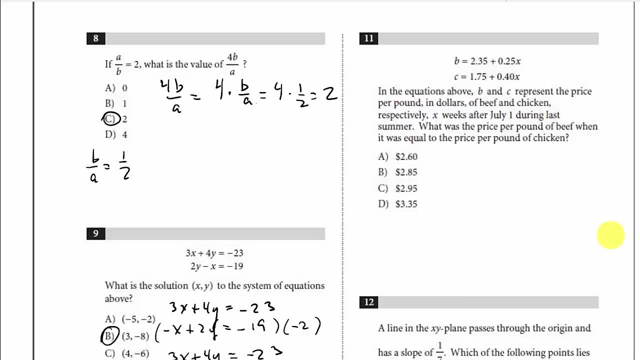 beef and chicken respectively x weeks after July 1st during last summer. What was the price per pound of beef when it was equal to the price per pound of chicken? All right, so we need to set these equal to each other. 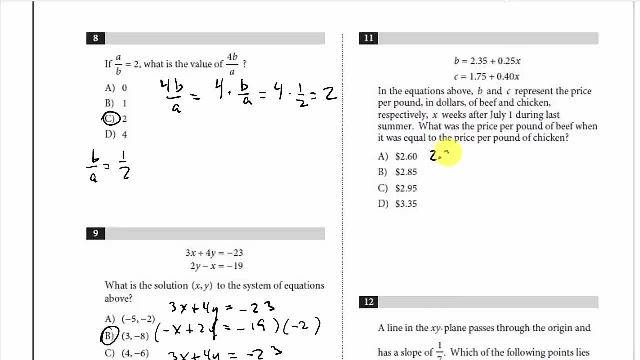 And so we can use시'll take g and solve for x. I'm going to want to go С and solve for g and solve for x. So that's going to be: 2.35 plus 0.25x is equal to 1.75 plus 0.40x. So we're solving an equation with decimals. Okay. Well, we want to get rid of the decimals because we can't use a calculator and it's a lot more difficult to do operations on decimals. So if we multiply the decimal numbers, we want to be able to solve for g and c here. 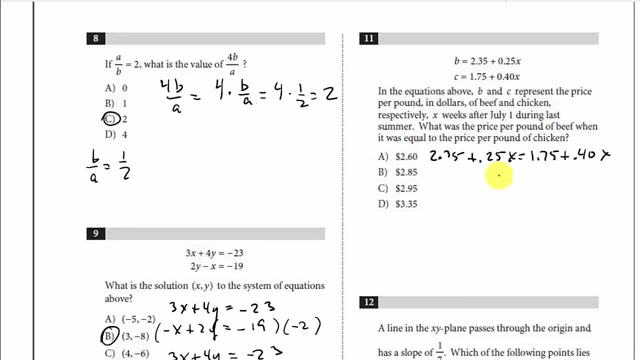 and it's a lot more difficult to do operations on decimals. so if we multiply, if we multiply each term by 100, because, see, we have to move the decimal two places to get rid of it, so that'll give us 235 plus 25 x plus 175 plus 40 x, and then we just solve, so we'll subtract 25 x to both sides. 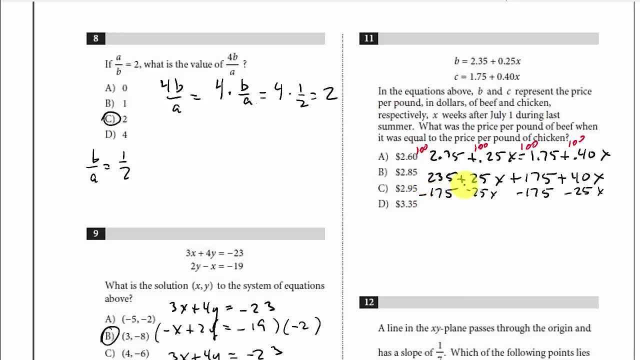 we'll subtract 175 to both sides, so that's going to give me: no, i'm sorry, this is 175. that should be an equal sign right there. so this is going to give me: 60 is equal to 15. x divide both sides by 15, i get x equal 4. but now what do we want to know? what is the price per? 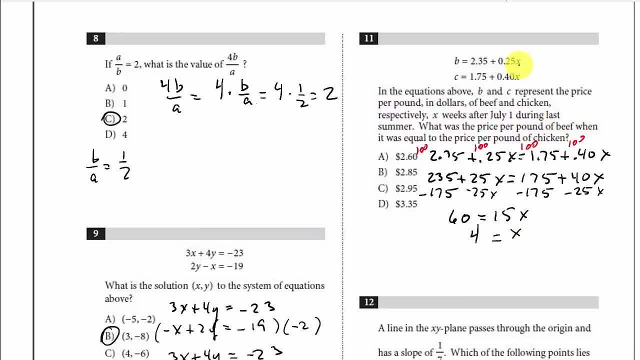 pound of beef. so we've got to take the x and plug it into here, so I get: B is equal to 2.35 plus 0.25 times 4. well, remember, 0.25 is the same as 1, 4th, and 1 4th times 4 is 1, and so that right. 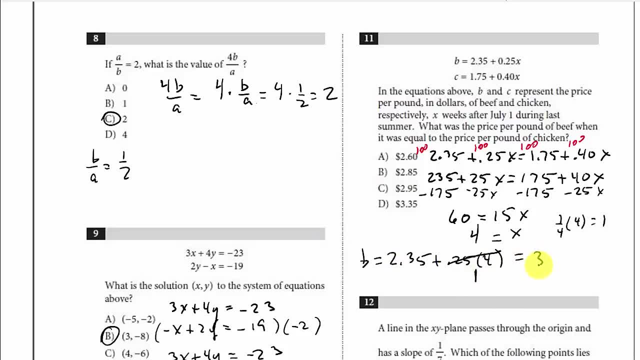 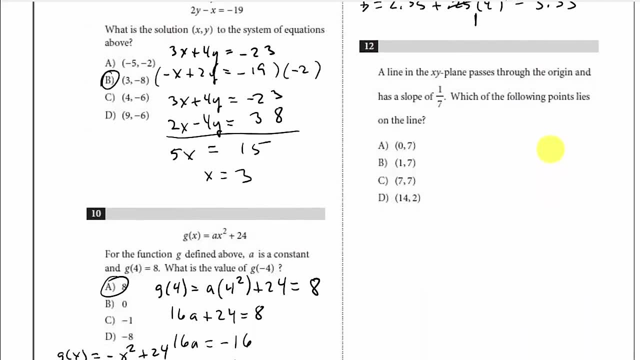 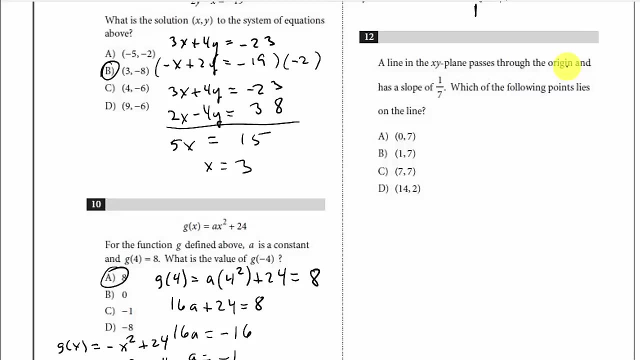 there is 1. this 2.35 plus 1 is 3.35, so that's D. all right, let's look at the next one. all right, it says a line in the XY plane passes through the, through the origin, and has a slope of 1: 7. which of the following points lies on the line? 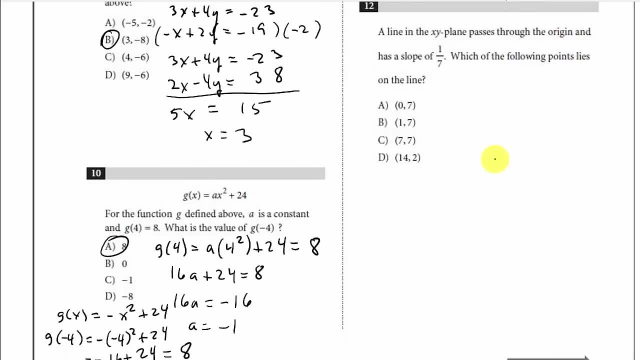 okay, so this one there. you know, there's a couple of ways we could probably do it, but I think the easiest way is if we just draw this and it tells us that it passes through the origin and we know that the slope is rise or run. so if we start here and we go up one unit and then we go to the right, 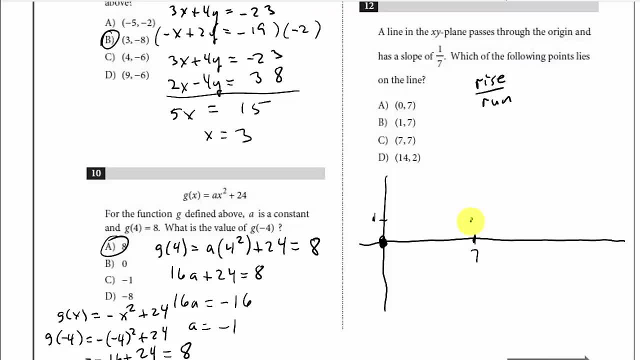 seven units. okay, that would be a point on the line. well, do you see the point? this would be what the 0.71? well, that's, that's not in here, so let's do it again. let's go up one more unit and then over seven units. so that would be. 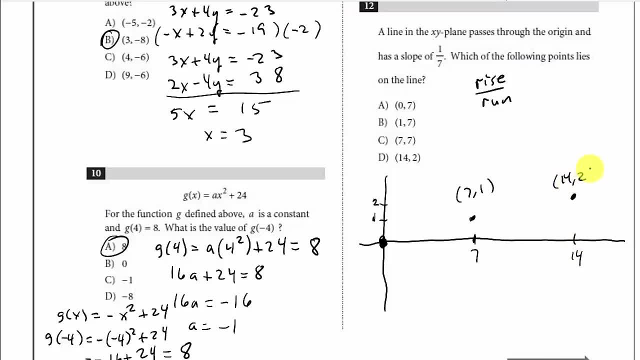 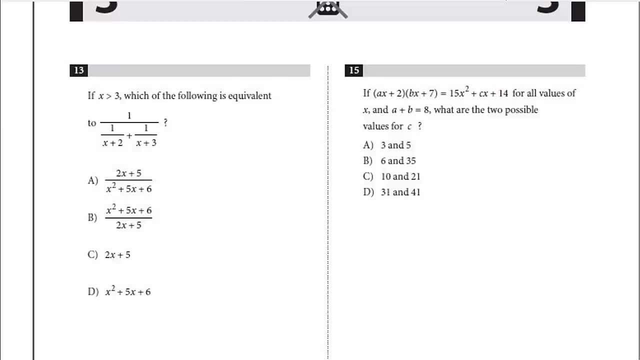 to 14. this would be the point 14. 2: well, you see, see it there. that's d. All right, so if x is greater than 3, which of the following is equivalent to this? So it looks like all they're doing here is they're just simplifying this. This is just. 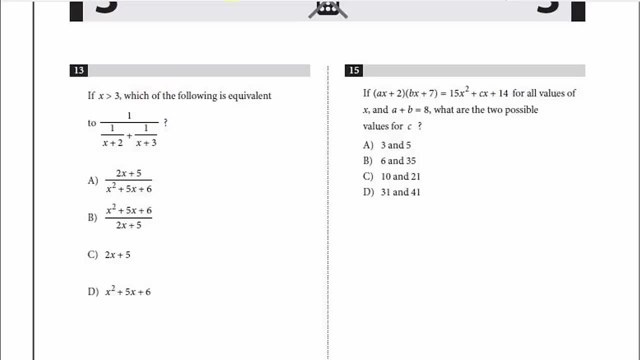 complex fractions. so we're going to multiply each term- see the 1,, this and this by the common denominator. Well, what's the common denominator? The common denominator is x plus 2 times x plus 3, and same thing here: x plus 2 times x plus 3, and x plus 2 times x plus 3.. Multiply each term. 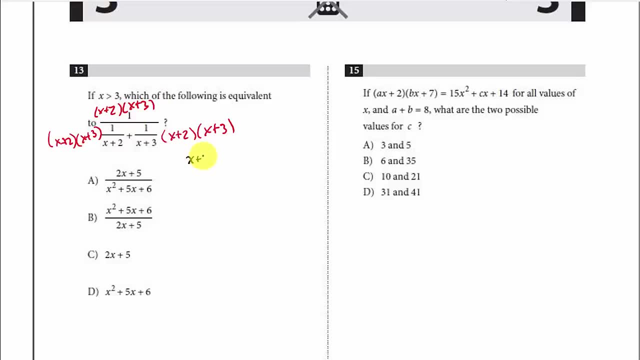 by the common denominator. So 1 times this, that leaves us with x plus 2 times x plus 3.. Here the x plus 2s cancel. So I'm left with just x plus 3.. Here the x plus 3s cancel. So 1 times that that's x plus 2.. 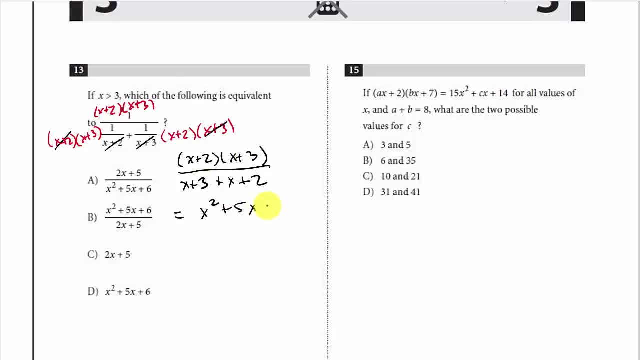 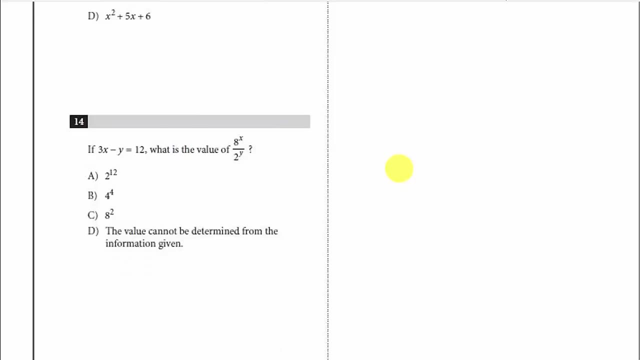 And so if I fold that, that's x squared plus 5x plus 6 over, and then x plus x is 2x and 3 plus 2 is 5.. And so that would be this one b. All right if 3x minus y equals 12,. 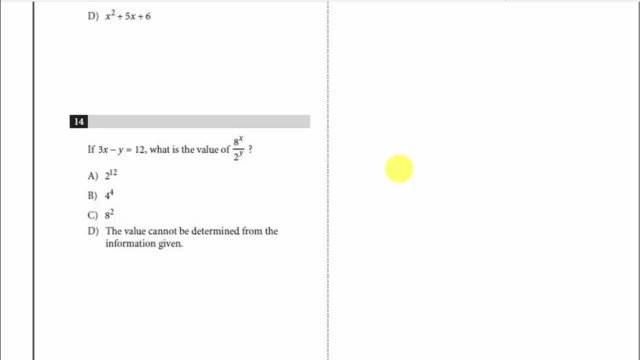 what is the value of 8x over 2y? All right, so this one's kind of tricky. I would be guessing. I would think that if you were guessing at this, you might guess d. But let's look at this. What we notice here about 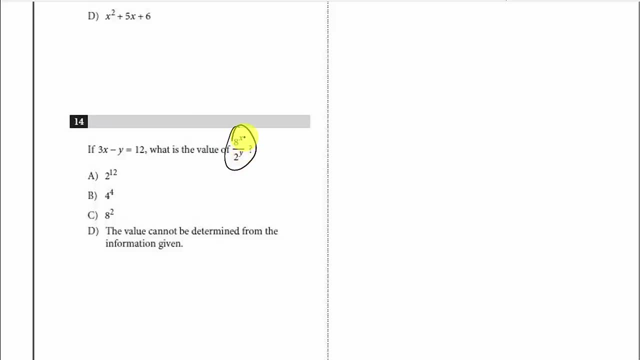 this is: this is 2 to the y and this is 8 to the x. Well, 8 can be written in terms of 2 raised to a power, 8 is 2 cubed, So let's just try that out and see what happens. And so I get 8 to the x. 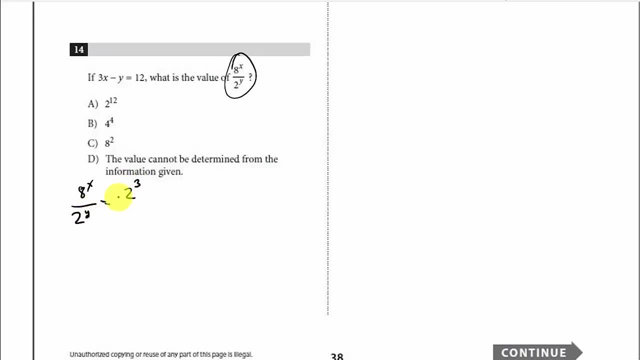 over 2 to the y. Well, 8 is what 2 cubed. And then that's raised to the x power over 2 to the y. And then- remember this, you multiply, So that's 2 to the 3x over 2 to the y. Well, remember. 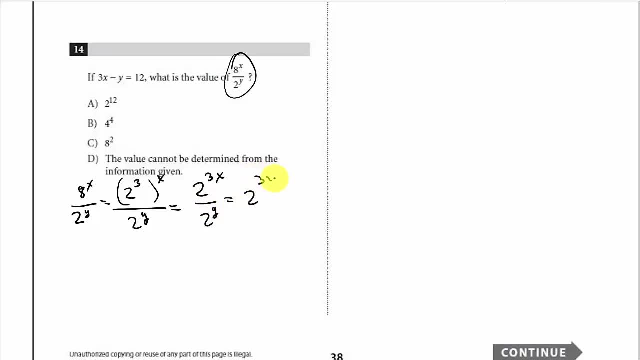 if you have like bases, what do you do? You subtract the exponents, So we get 2 to the 3x minus y, So this is equal to 2. Well, that's 3x minus y. Well, they told us up here it's 12.. And so this would be a. 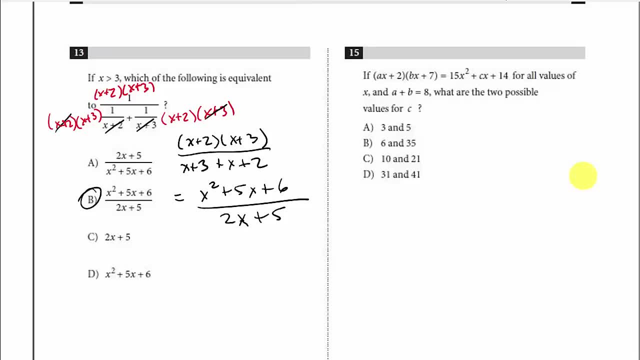 All right. so here, if ax plus 2 times bx plus 7 equals 15x squared plus cx plus 14, for all values of x and a plus b is equal to 8, what are the two possible values of c? this value here. 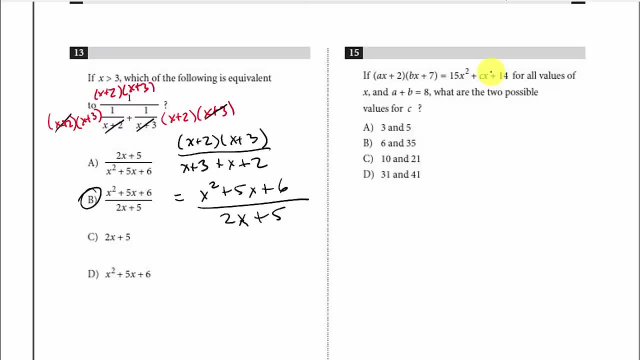 All right. so let's take a look at this. Let's set this: Okay. well, we got this equal to this, So we've got ax plus 2 times bx plus 7 equals 15x squared plus cx plus 14.. Well, let's go ahead and multiply this out, So that's abx squared. 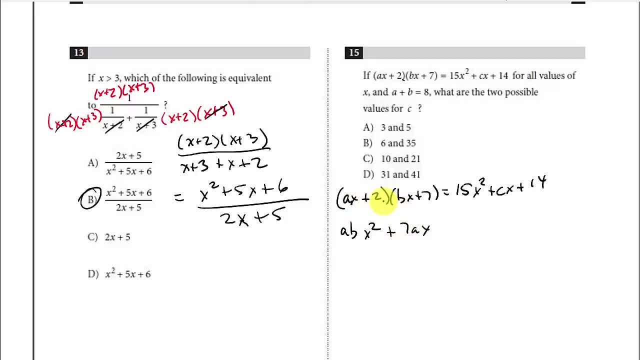 the first and then the outside plus 7ax, the inside plus 2bx and then the last plus 14, is equal to 15x squared plus cx plus 14.. So this is abx squared plus, and what I'm going to do here is: 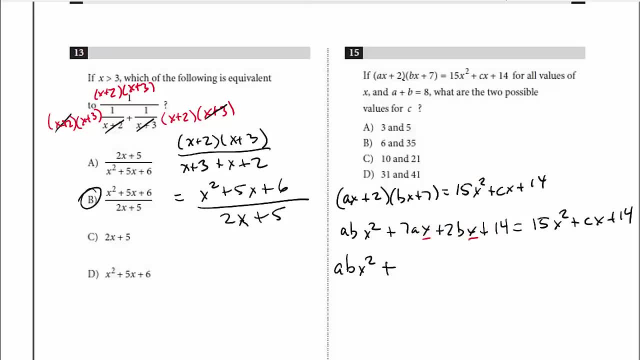 I'm going to factor out this common factor of x, and so that's going to be 7a plus 2b. I don't know if it'll help or not, but we're going to see Equals 15x squared plus cx plus 14.. 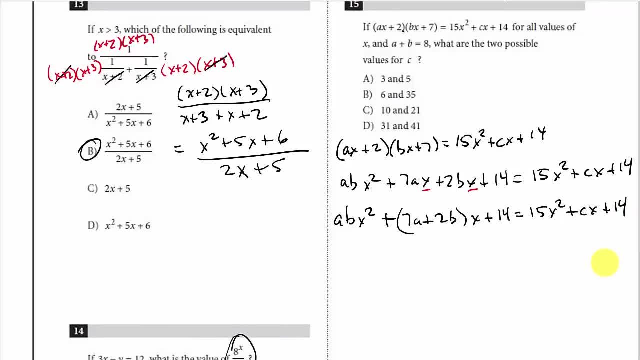 All right, so let's see what we've got. Well, let's see what we know. We know that ab- let me do this in a different color- We know that ab is equal to 15, because see the x squared and the 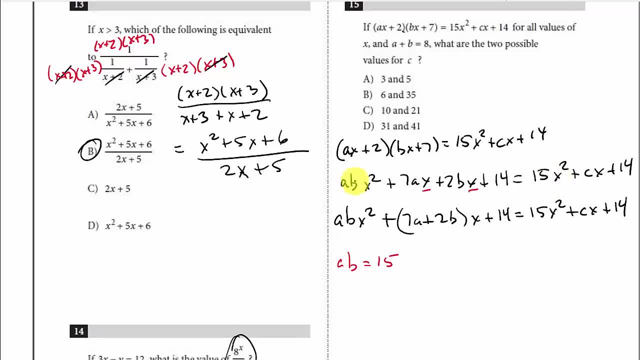 x squared. the coefficient of this x squared is 15, so a times b has to be 15.. Okay, all right, let's see what else we've got here. Well, they tell us up here that a plus b is equal to 8,. 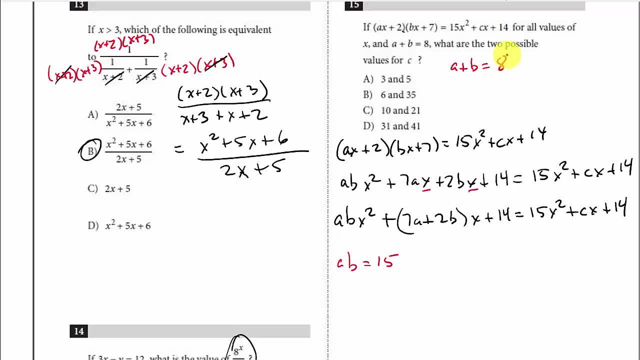 right. So we know. let's see what we know here. Well, that tells us that b is equal to 8 minus a, so I could actually take this and plug it in for b, So I've got a times 8 minus. 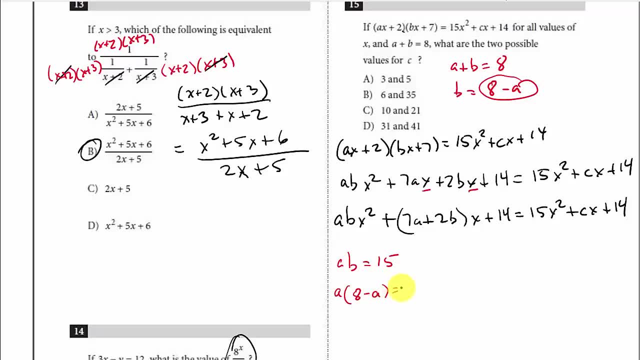 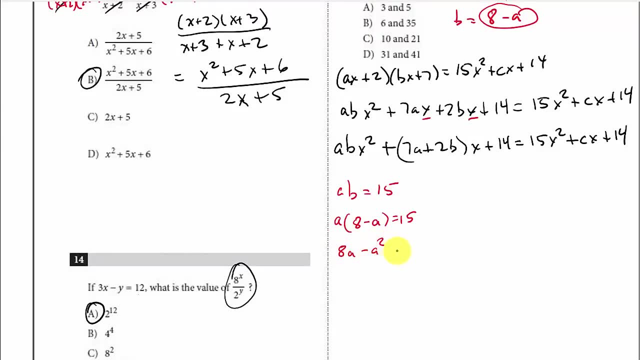 whoop, I'm sorry. 8 minus a is equal to 15, and so that's going to give me 8a minus a squared equals 15, and then, if I move these over to the other side, that's going to give me a positive, a squared. 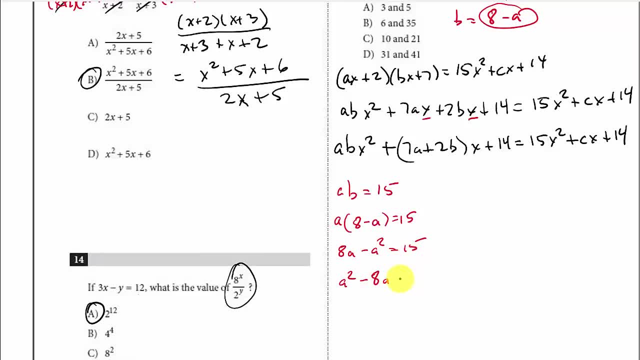 Move this over. that's going to give me minus 8a and that just stays on the same side: 15, and instead of putting the equal zero over here, I'm going to put the equal zero over here. All right, so now let's just. 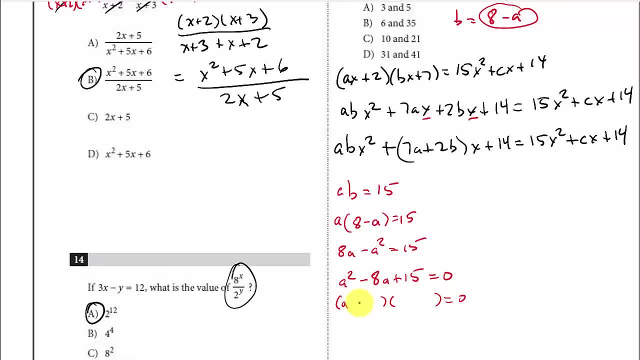 let's factor this, see what happens. So let's see that's going to be what: a minus 5, a minus 3, set each one equal to zero, and so a equals 5, or a equals 3.. All right, so now? well, we can figure out what c is, because we know that c. 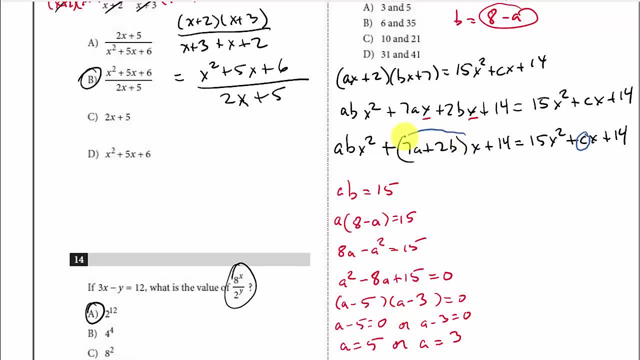 is the coefficient of x, and so we know that c is the coefficient of x, and so we know that c is the coefficient of x, and this is the coefficient of x over here and we can plug in for a and b. You see that. 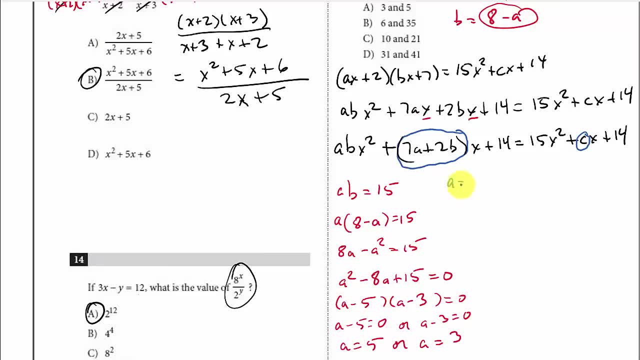 So look at this: When a is equal to 5, that means b is equal to what? Well, we plug the 5 into here. 8 minus 5 is 3, and then, when a is equal to 3, we plug that. 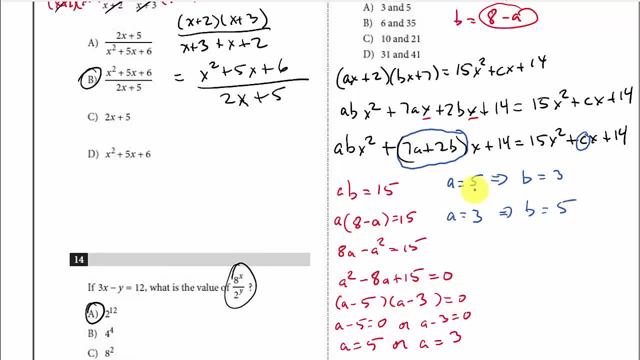 and that gives us b is equal to 5.. So let's do this one first, So I get 7 times 5 plus 2 times 3, and that is equal to 41.. So c could be 41, and then we let's plug this one in, so 7 times 3 plus. 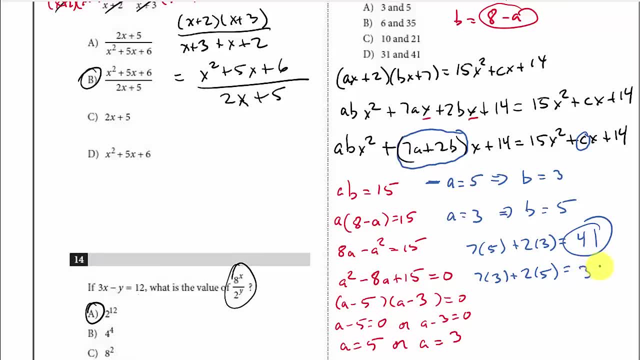 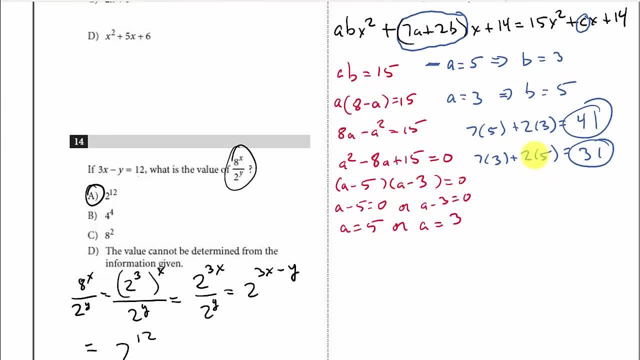 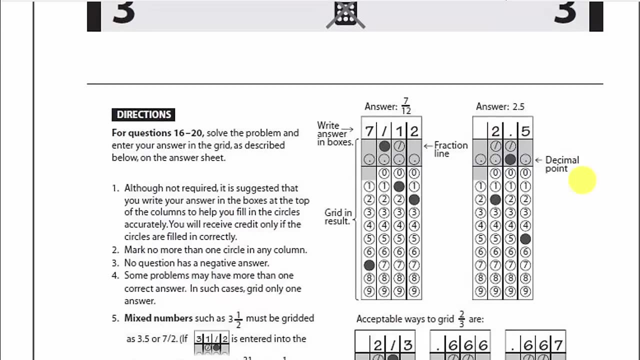 2 times 5,, well, that equals 31.. So c could be 41, or 31,, and you can see that is d. All right, so this page here, this just kind of tells you directions on how to fill out your. 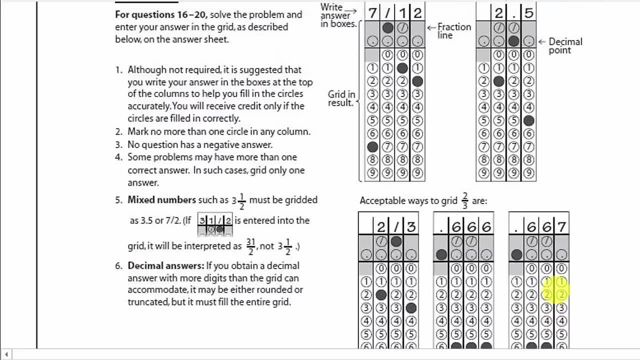 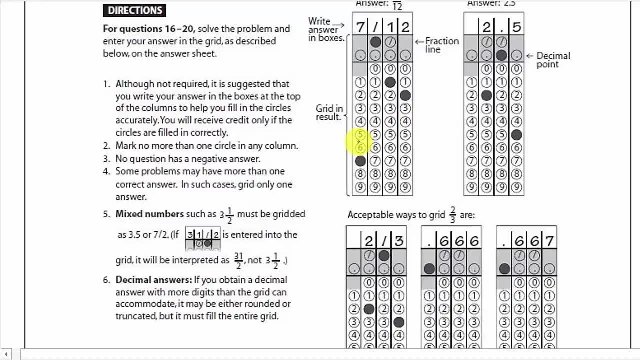 answers for the last page. I'm not going to come back and fill my answers out on- you know, a page like this. I'm just going to work the problems and give you the answers. So let's just go on to the next page and work those problems. All right, so all right. 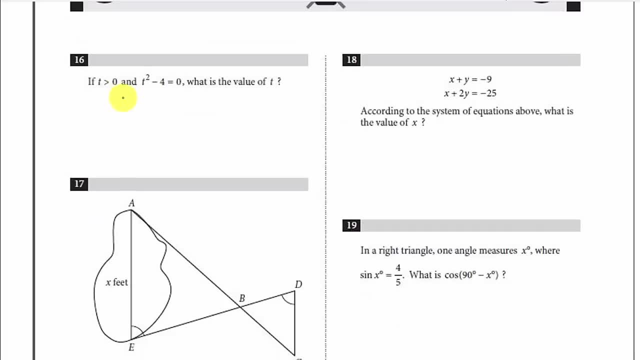 so we're down to the next page. So we're down to the next page. So we're down to the next page. So we're down to the last five problems. All right, so if t is greater than 0, and t squared. 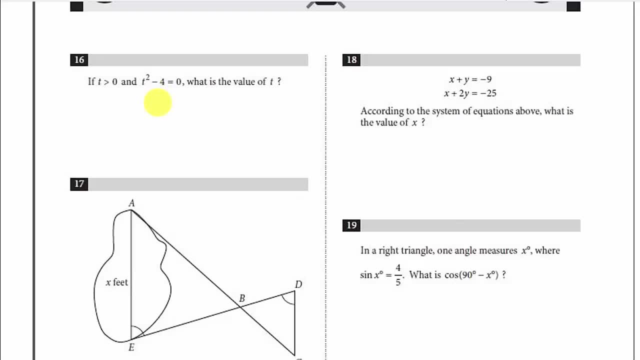 minus 4 is equal to 0,. what is the value of t? All right, so well. we just solved this. We moved the 4 over. t squared equals 4.. So remember the square root property: t is equal to plus or. 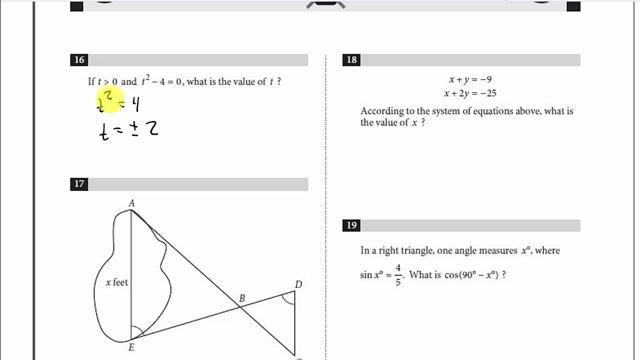 minus 2.. Don't forget to put the plus or minus 2.. But they do tell us that t is greater than 0, so they don't want the negative, They just want the positive. okay, And the reason? I tell you not. 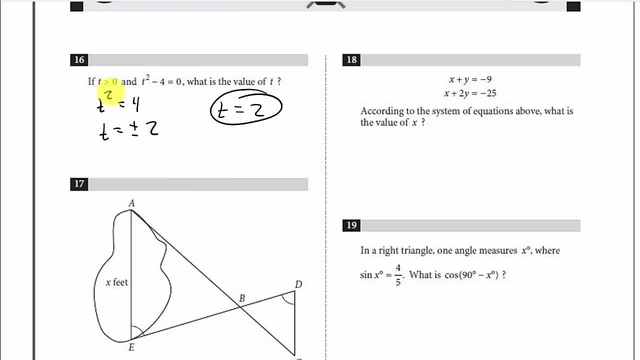 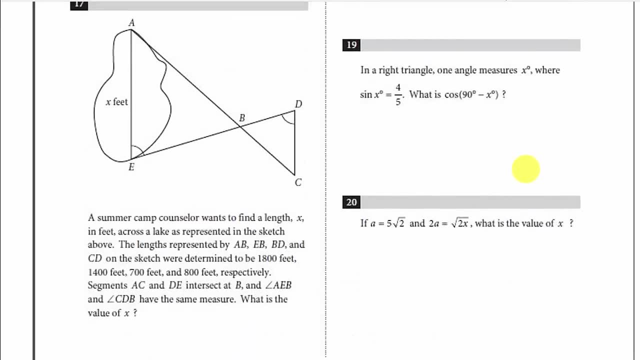 to plug that in is because you don't want to plug that in. You don't want to plug that in, You forget the plus or minus is because on the test they may say t is less than 0. And then you would choose the negative 2.. All right, so let's look at this one. It says a summer camp counselor wants. 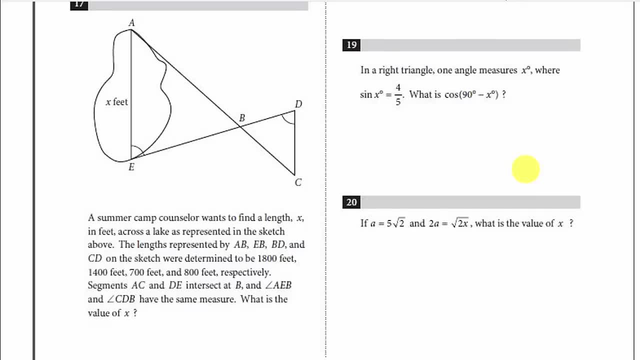 to find a length x in feet across a lake as represented in the sketch above. The lengths represented by a, b, e, b, b, d and c d on the sketch are determined to be 1,800,, 1,400,, 700,. 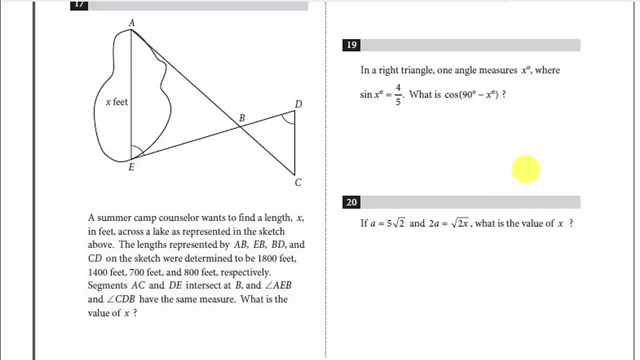 and 800. feet respectively. Segments a, c and d- e intersect at b, and angle a, e, b and c, d, b have the same measure. What is the value of x? All right, so let's just start out first by labeling. 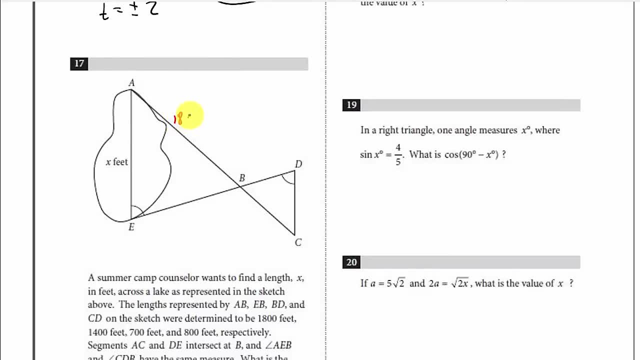 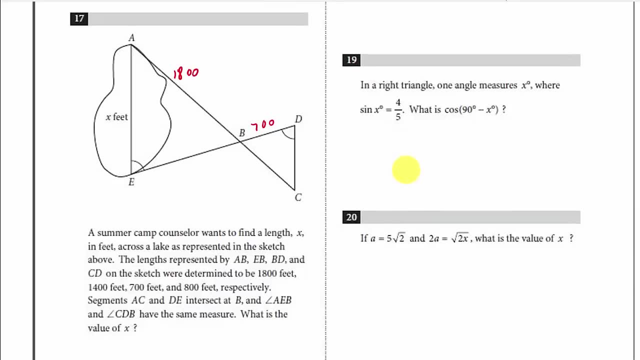 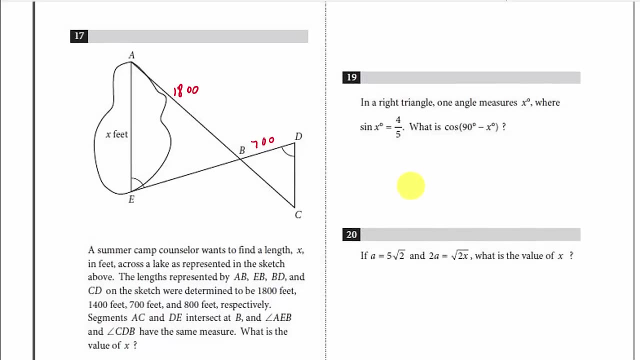 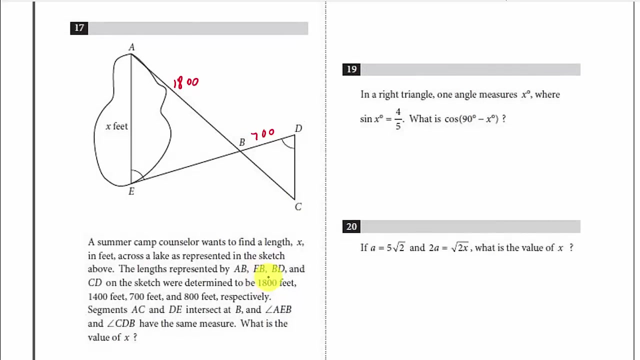 this thing. So this is 1,800.. This is 700.. Is that right? B d, Yeah, So that's going to be 700. And then e b do they tell us that, Yeah, that's 1,400.. And then they: 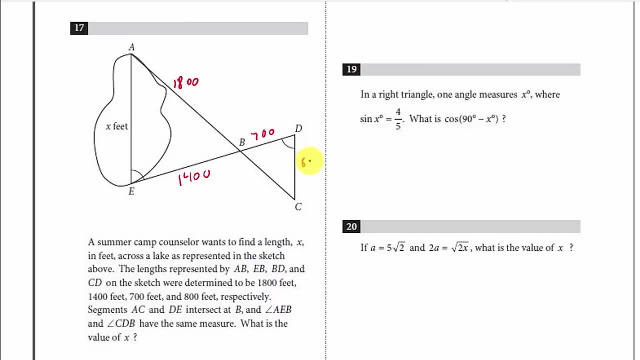 give us c, d. Well, that's 800.. All right, What is the value of x? So we're looking for this value Here. All right, So we know that this angle and this angle are the same. So all this is. 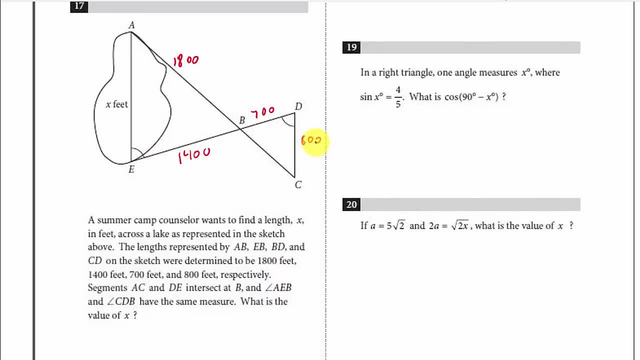 this is just a proportion. So we can say c over d, So c over d over x, this side, Okay. So these would be similar triangles. Okay, These are similar triangles. This angle and this angle are the same, And then that would equal what? B d, B, d over e b? Okay, So this side is proportional to this. 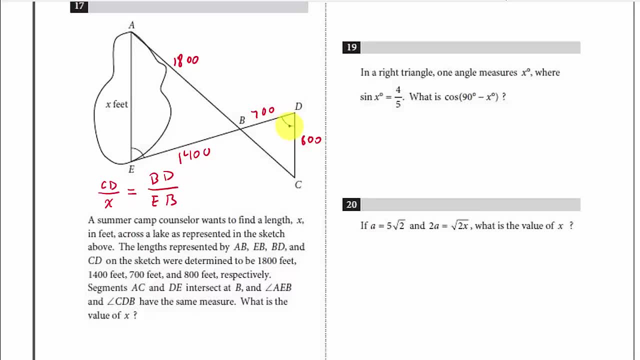 side. Okay, Because they see they give us these angles here are similar. So now it's just a matter of plugging all this in. So that's just going to be what 800 over x equals c over d. So that's just going to be what 800 over x equals c over d. So that's just going. 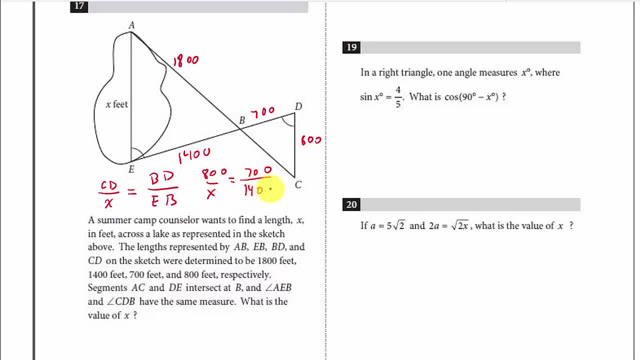 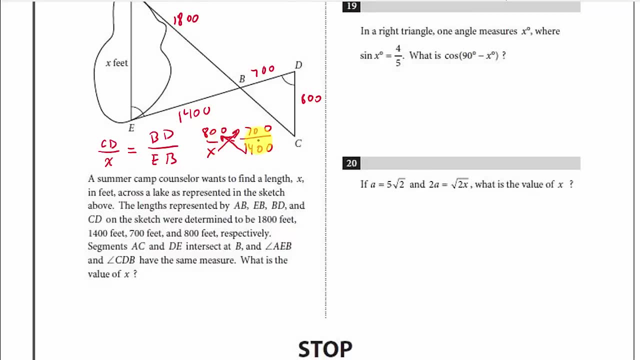 to be what: 800 over x equals 700 over 1400.. So if I move the x up here, the 1400 goes up there. So that's going to be: 800 times 1400 is equal to 700 x. Now look, don't multiply that out, They're. 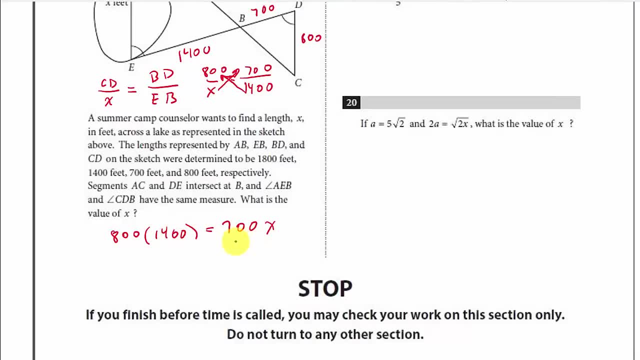 not letting you use a calculator, So they're probably not going to give you very difficult problems to add and multiply and subtract. So we divide by 700 on each side. Look, that goes in, That's two, So that 1600 is equal to x. And so there's your answer. 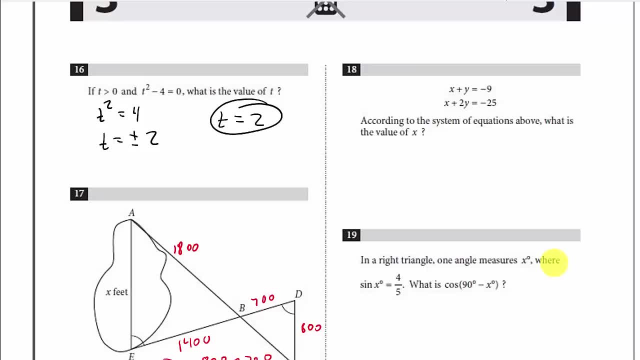 All right, According to the system of equations above, what is the value of x? All right, So well. just, we did one of these a while ago, Let's just go ahead and make. Alright, so they just want to know the value of x, so okay. so let's get rid of the y terms. 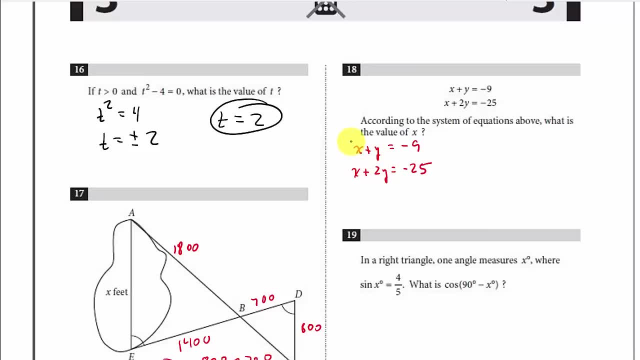 and then we can solve for x. So to do that we're just going to need to multiply this one by negative 2.. Okay, I know it would be easier just to subtract the 2, and the x's would go out. but then we 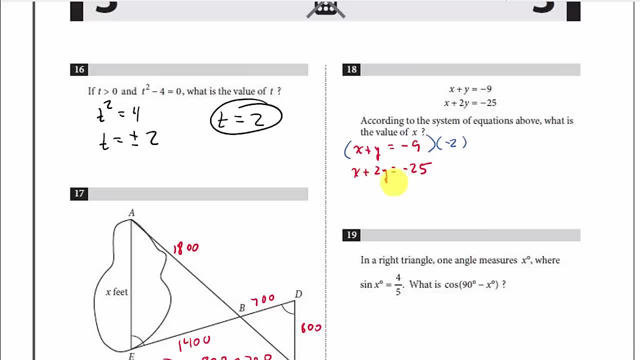 would solve for y, and then we would have to plug that back in to get x. So let's just eliminate the y's, Alright. so that's going to be negative. 2x minus 2y equals 18, and x plus 2y equals negative. 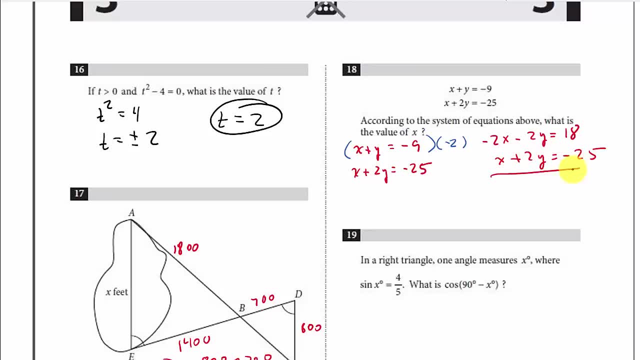 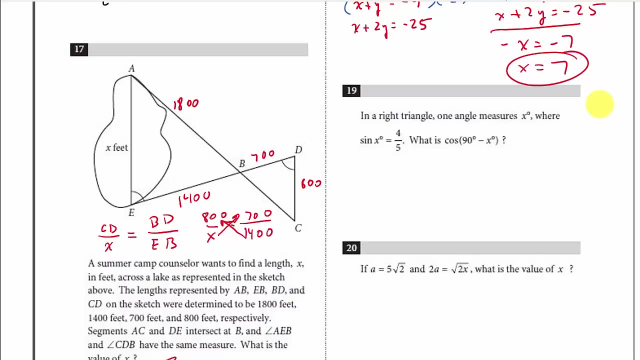 25.. And so that's going to give me negative x equals negative 7 divided by negative 1, x equals 7.. In a right triangle, one angle, measures x naught, where the sine- I mean measures x degrees. where the sine of x degrees is 4 fifths, what is cosine of 90 minus x degrees?